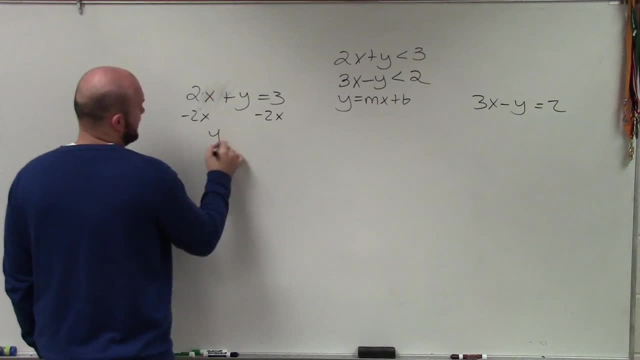 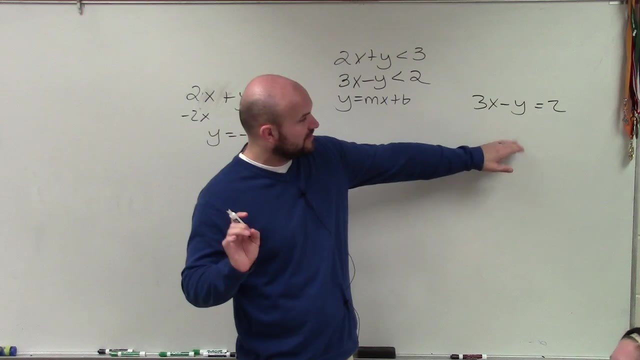 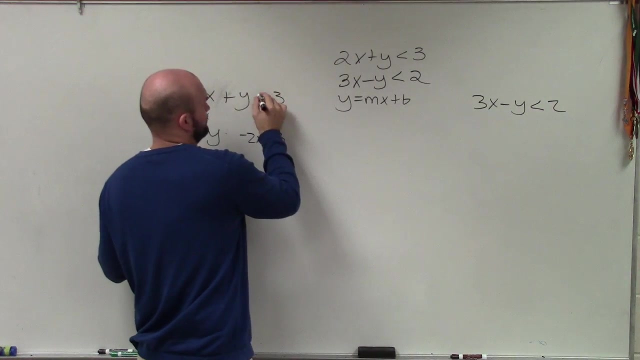 form. So to do that, I subtract 2x on both sides and I get y equals negative 2x plus 3.. Over here, it's very, very important for us to understand. I'm actually going to leave my inequality left there. I don't actually know why I changed that. So here I subtract 3x. 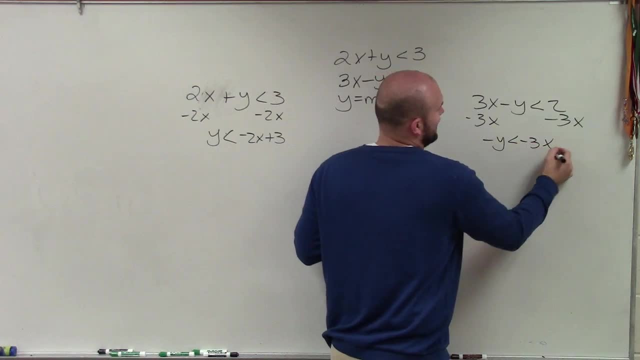 and I have negative y is less than negative 3x plus 2.. Now notice, ladies and gentlemen, I am now going to be able to solve for y. I'm going to subtract 2x on both sides and I'm going to be dividing by negative 1.. Remember, whenever we divide, we flip our inequality. 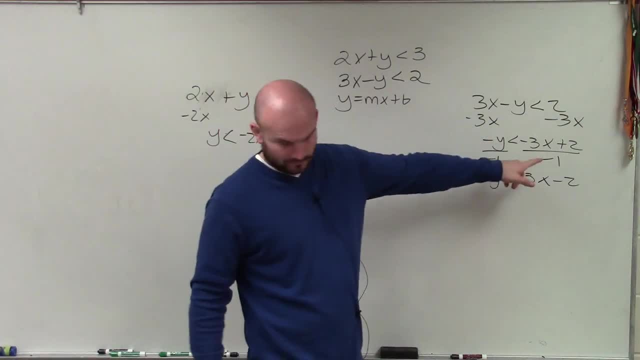 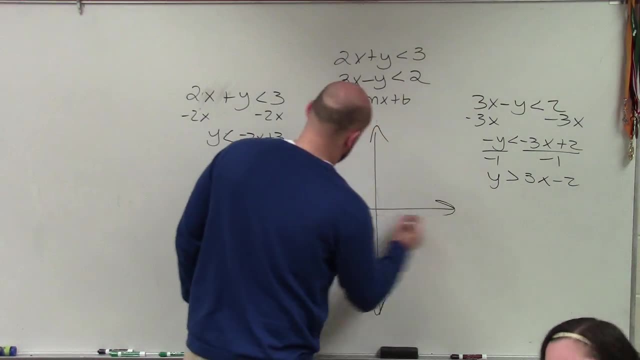 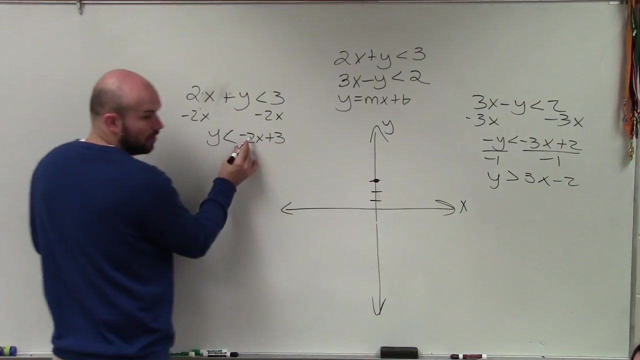 symbol. right, You divide it because you don't want y to be negative. Yeah, solve for y is positive. Now we just identify our slope and our y-intercept. Here my y-intercept is 3, so on the y-axis I go up to 3.. 1,, 2,, 3.. My slope is negative, 2.. 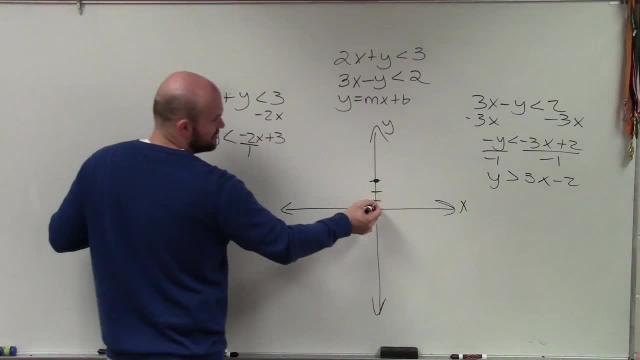 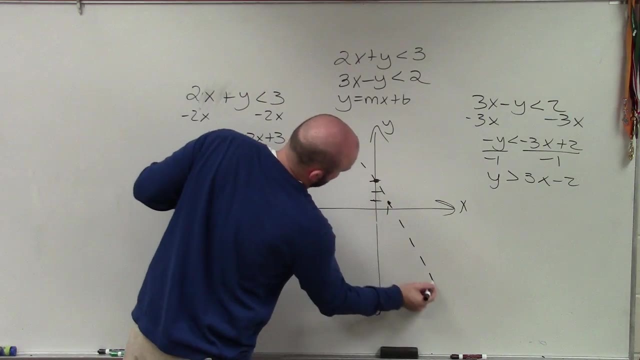 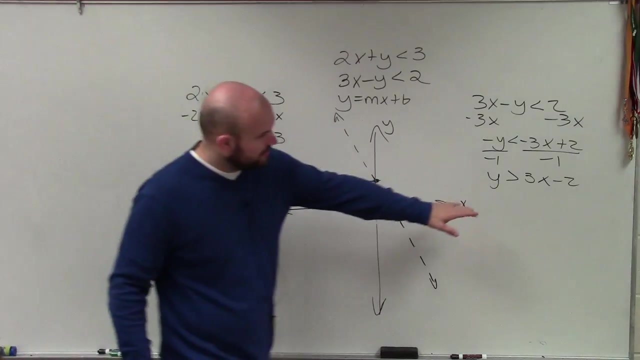 We always want to write our slope as a fraction, so that's going to be down 2. Over 1.. Notice that this is less than so. I'm going to have a dashed line. Now we go ahead and go to this one. This one has a y-intercept of negative 2.. Make a point. Now my slope. 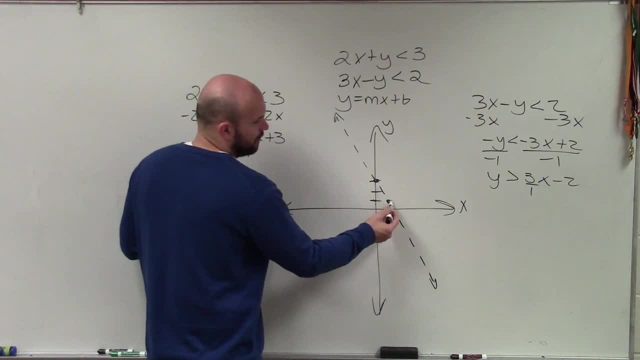 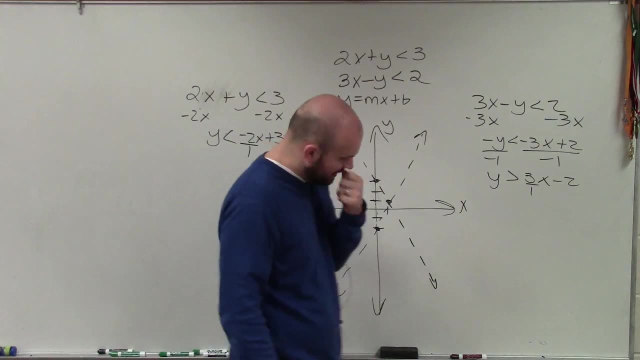 here is 3 over 1, so I'm going to go up 3 over 1.. Notice that's greater than so again, that's going to be a dashed line. Now, ladies and gentlemen, what we're going to be looking at is applying our test points. 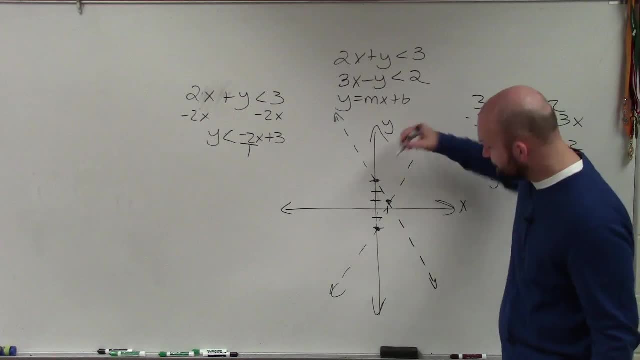 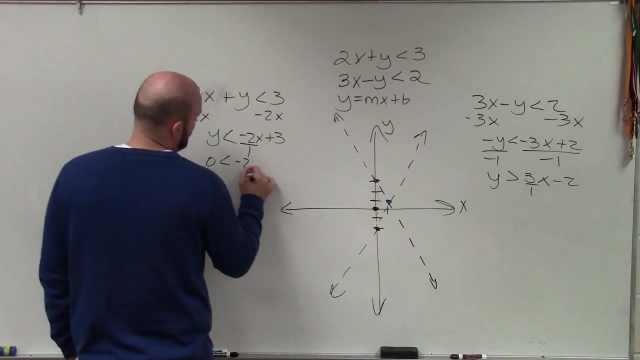 To do that we need to determine a point that we can help us shade. The best point to always pick, that is, as long as it's not on your lines, is 0, 0.. I plug in 0 in for x and 0. 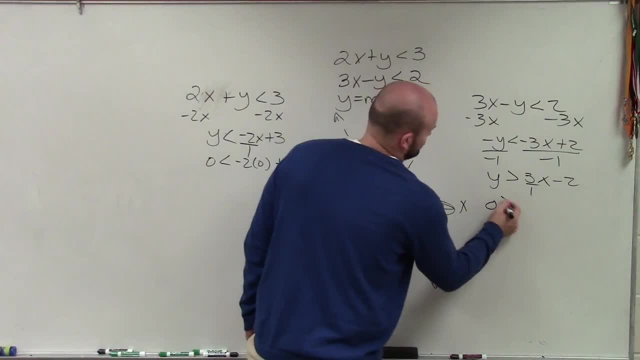 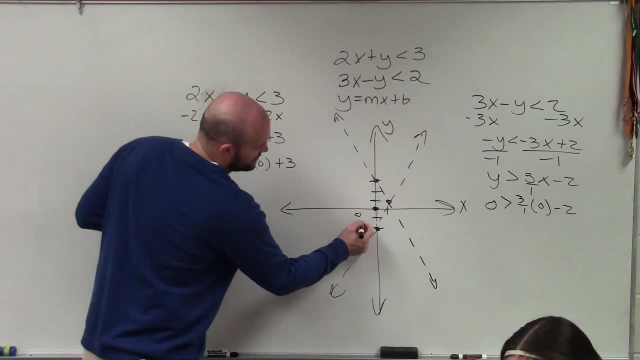 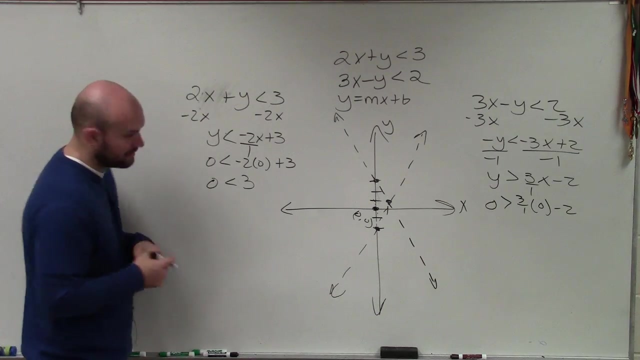 in for y For this equation because, remember this point- 0, 0 has an x and a y coordinate of 0, 0. So therefore I have: 0 is less than 3.. Is that true or false? 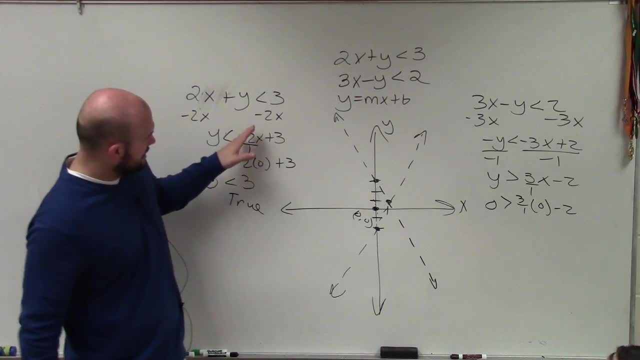 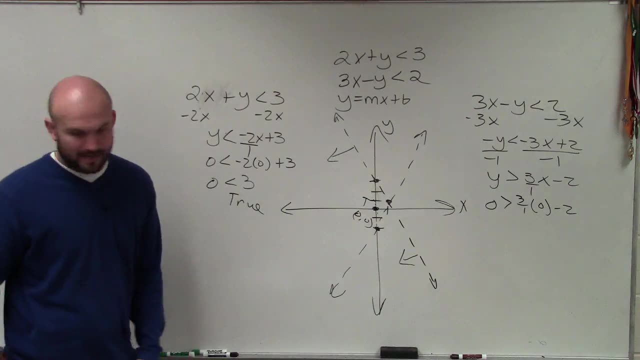 True. So that was this equation. Since that's true for this equation, I'm going to shade towards the test point. Now we're going to try this one: 0 is greater than negative 2.. Is that true or false? 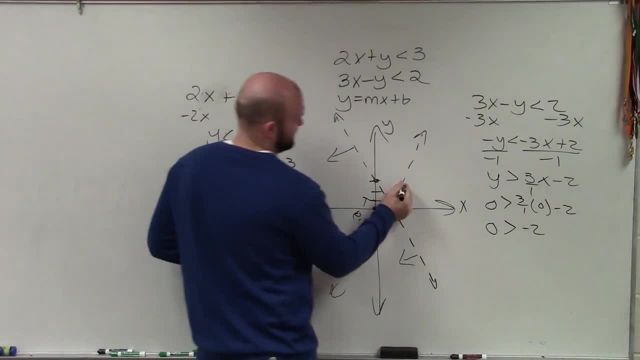 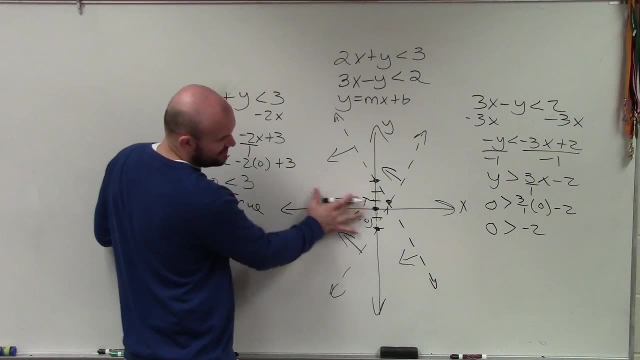 False, True, True, True, I'm sorry. So again, we're going to shade towards the true points. You can see that this region is where it's true for both inequalities. So that is where I'm going to shade. 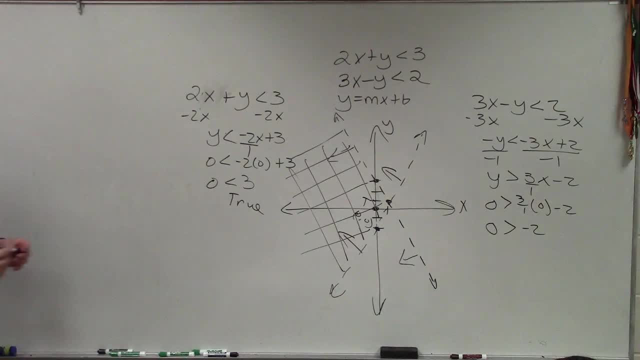 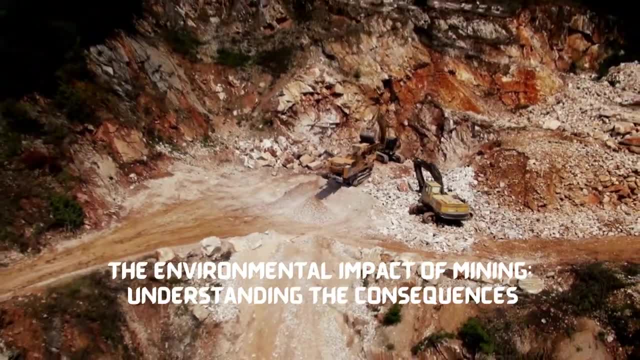 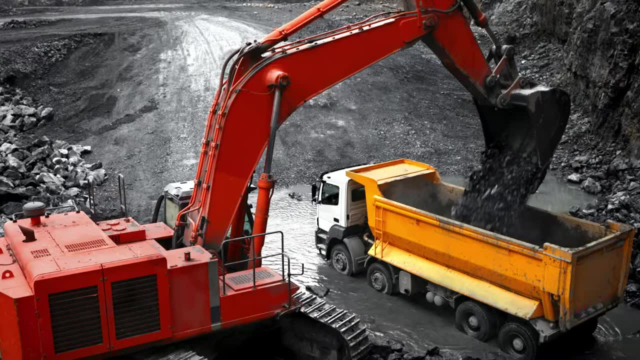 Mining has been a part of human civilization for thousands of years, providing us with the raw materials we need to build our homes, cars and electronics. But what many of us don't realize is the devastating impact that mining can have on the environment. One of the most common 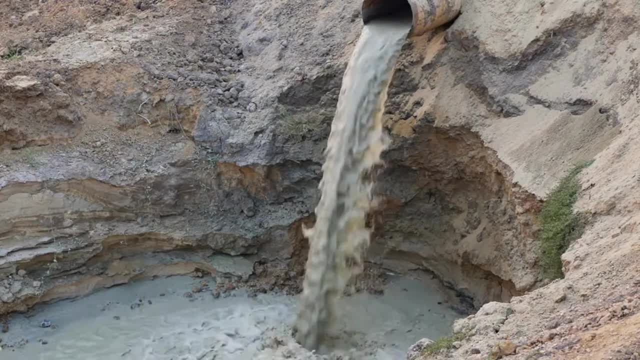 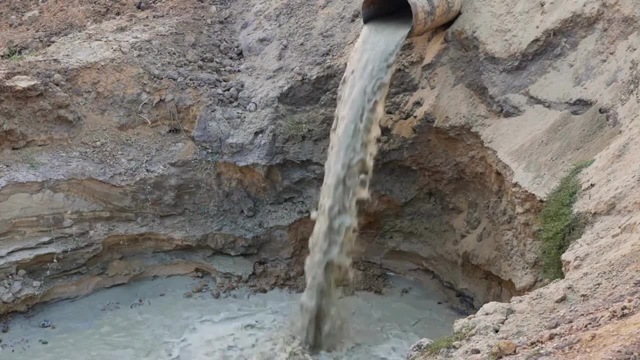 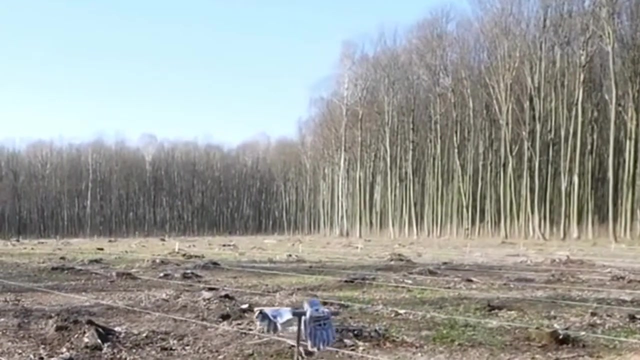 environmental impacts of mining is water pollution. When minerals are extracted from the earth, they often release harmful chemicals and heavy metals into nearby rivers and streams, contaminating the water and harming aquatic life. Mining also contributes to deforestation, as large areas of forest are often cleared to make way for mining operations. 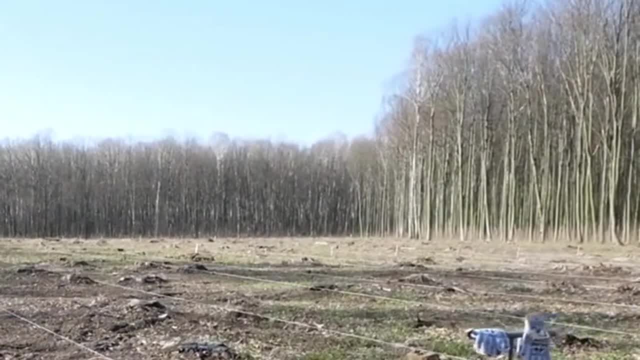 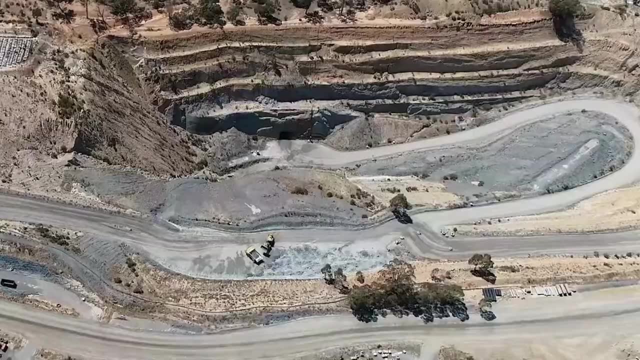 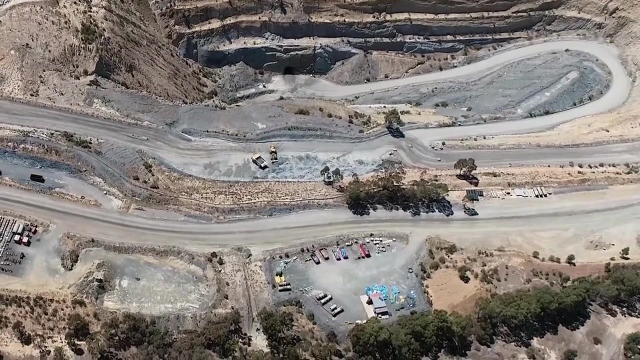 This not only destroys important wildlife habitats, but also increases the amount of carbon dioxide in the atmosphere, contributing to climate change. Another major impact of mining is the creation of toxic waste. When minerals are processed, large amounts of waste rock and tailings are generated, which can contain harmful chemicals.